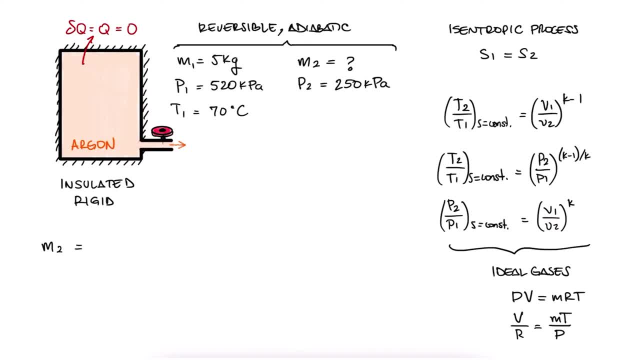 2 and argon is an ideal gas. Since the volumes and R didn't change, we have that M1T1 over P1 is equal to M2T2 over P2 and therefore M2 is equal to M1T1P2 over P1T2.. 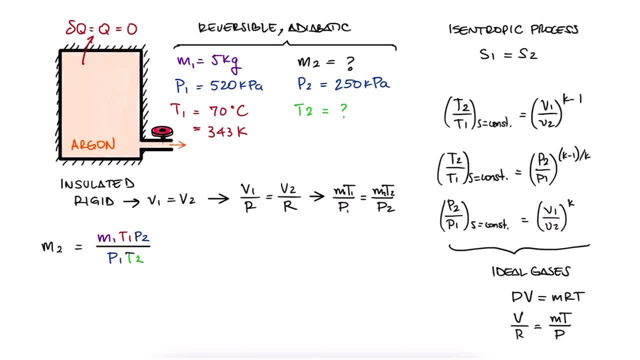 We have all the values except for T2.. This means that the relation that we derived in the main lecture video that we need here is the one that relates temperatures and pressures, because we do have the pressures From this expression, we solve for T2 and notice that we need the K ratio, Cp over Cv. 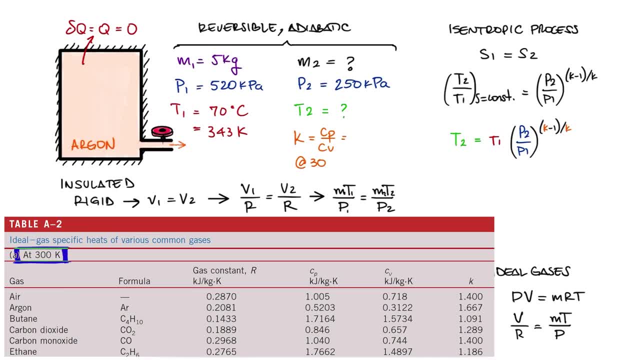 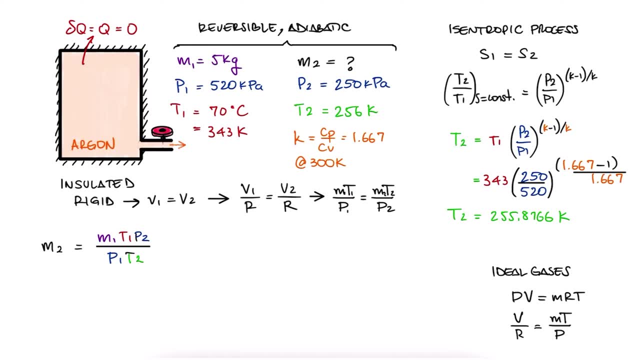 Since we don't know what the final temperature is gonna be, we can assume 300 Kelvin for now to get K and substitute the values with T1 and Kelvin to find T2. Since with this value for T2 and T1, we would get an average of 300 Kelvin anyways, our 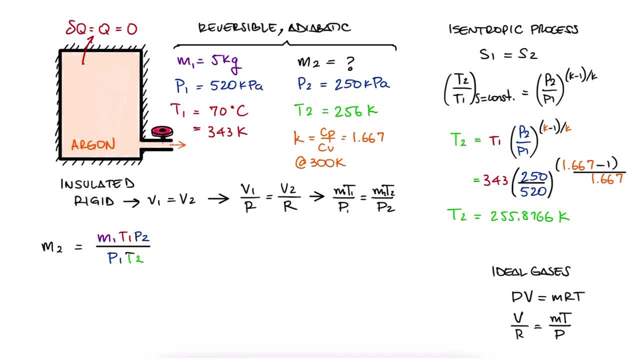 K value is on point. If this wasn't the case, we would iterate by taking the new K value for T1 and T2.. Now we can calculate for the average temperature and calculate 2 again and repeat this process until the temperature converges. 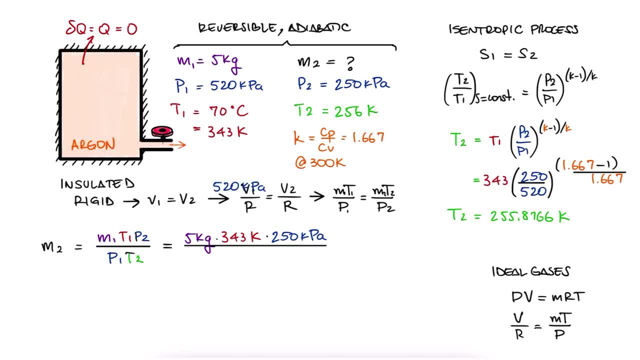 We now go back to our mass equation, substitute all values once again in Kelvin and find the value for M2, the mass at the end of the process. If you want to check out other examples for the reference entropy and specific heat topic, 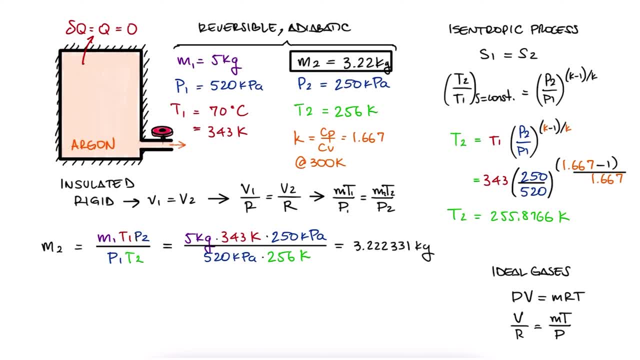 make sure to check out the links I left down in the description below, where you'll also find the links to the other lectures of the thermodynamics course. You'll also find the playlist. Thanks for watching. 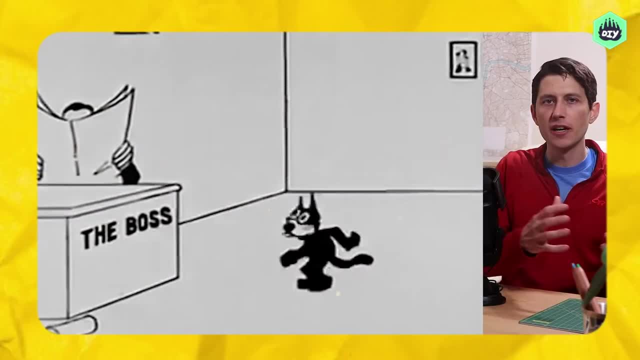 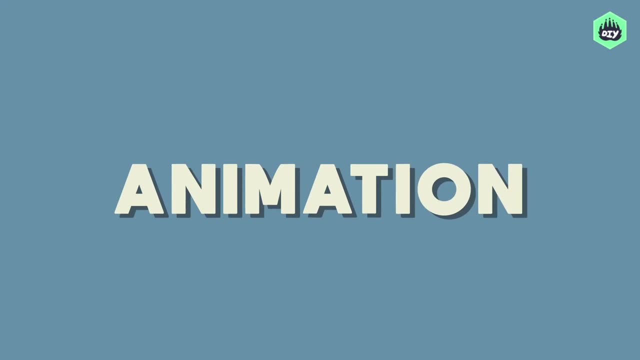 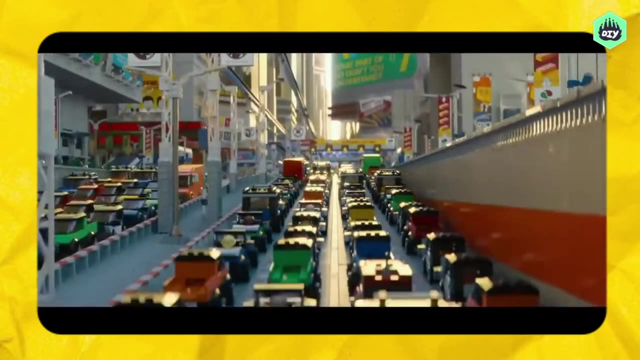 Tell me something that's so fun you don't even realize you're picking up problem solving and technical skills, while also boosting your imagination. It's animation, of course. Join animator Lucas Ridley, who's created content for brands like Lego and worked on films like Avengers, The Infinity Wars, and get started on animating your ideas to life. 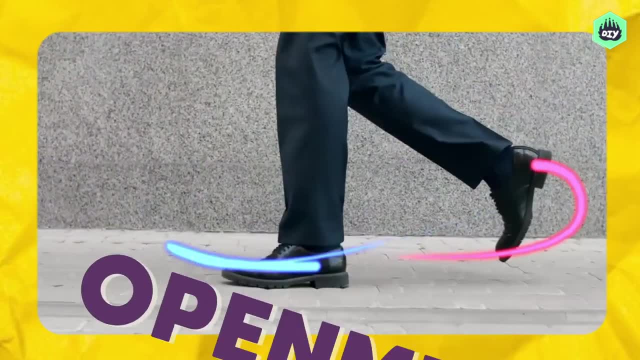 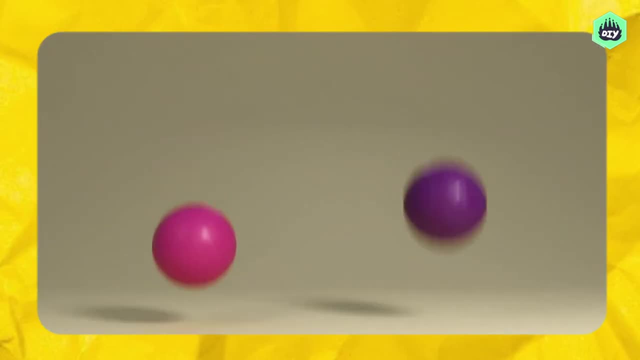 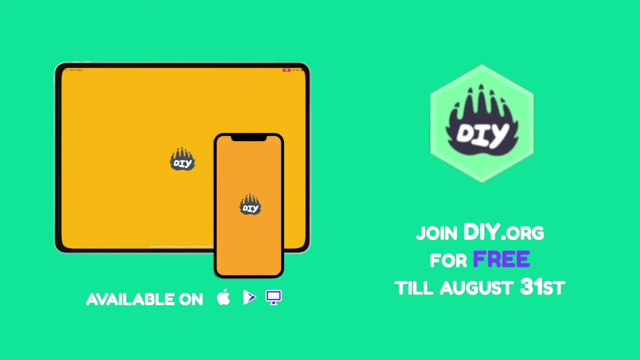 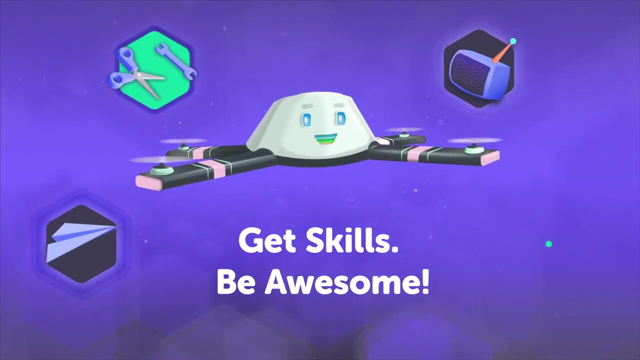 All you gotta do is bring an open mind and a whole lot of passion to the table. You'll be making awesome zip-flop books and smooth stop-motion videos in no time. Ready, Let's go. Oh hey there. Head on over to DIYorg for fun projects, how-to videos, TV shows and a global community of kids just like you.